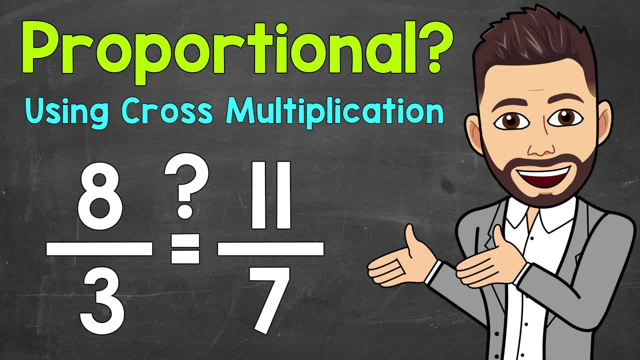 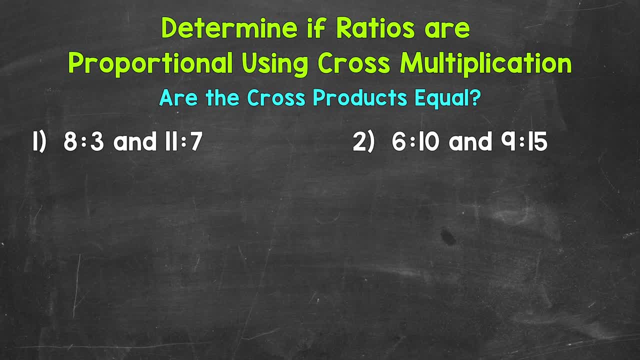 Welcome to Math with Mr J. In this video, I'm going to cover how to determine if two ratios form a proportion using cross-multiplication. Now remember: a proportion is formed by equal or equivalent ratios. In other words, equal or equivalent ratios are proportional. 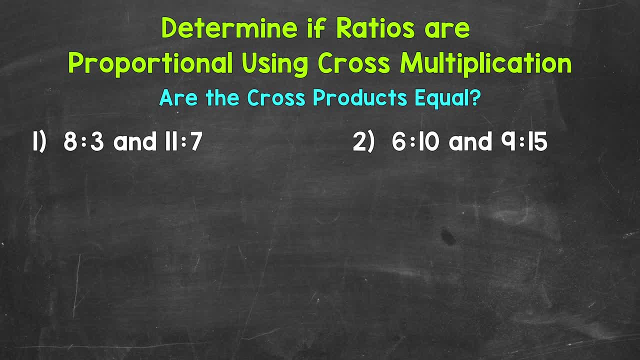 Let's jump into number 1, where we have 8 to 3 and 11 to 7.. Now, when it comes to checking if two ratios form a proportion using cross-multiplication, all we need to do is cross-multiply and see if our cross-products- the numbers we get once we multiply- are equal or not. 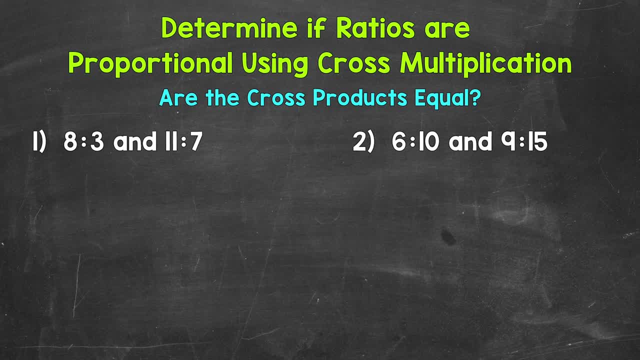 If they are equal, then we have a proportion. If they are not equal, then we do not have a proportion. Let's start by setting our ratios up in fractional form and setting them equal to each other. Now they may not turn out to be equal, but for now, set them up as a proportion. 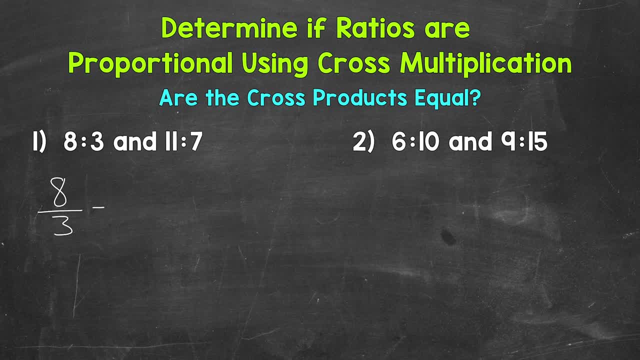 We have 8 to 3 and 11 to 7.. Now we can cross-multiply, so we multiply diagonally. We'll start with 8 times 7.. So 8 times 7. And then bring our equal sign straight down. 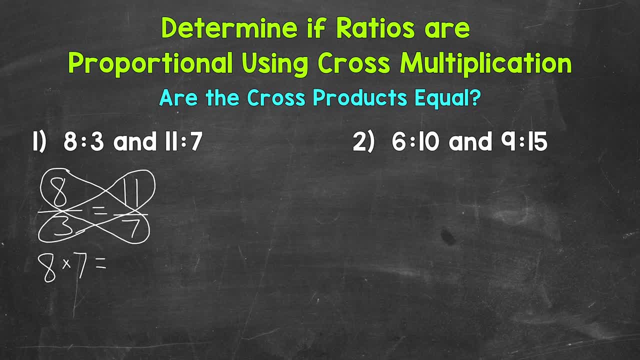 And now we can do 3 times 11.. 8 times 7 is 56.. 3 times 11 is 33.. 56 is not equal to 33.. So our cross-products were not equal. That means we do not have a proportion. 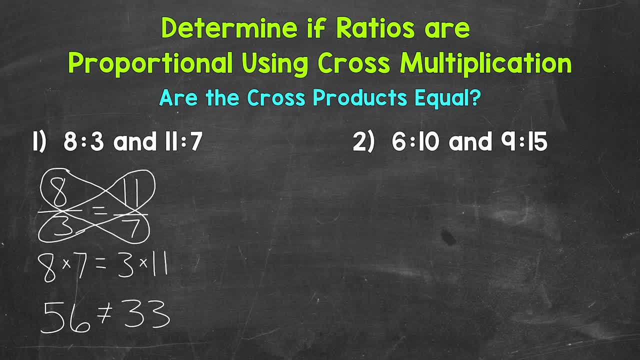 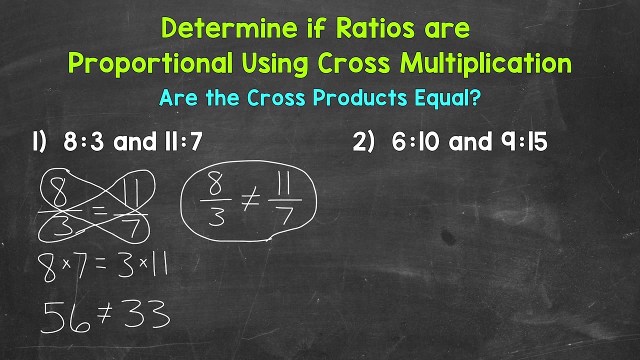 8 to 3 and 11 to 7 are not proportional. They do not form a proportion. So we can write this out as 8 to 3 is not equal or not proportional to 11 to 7.. Now one more thing I do want to mention about cross-multiplying these ratios.